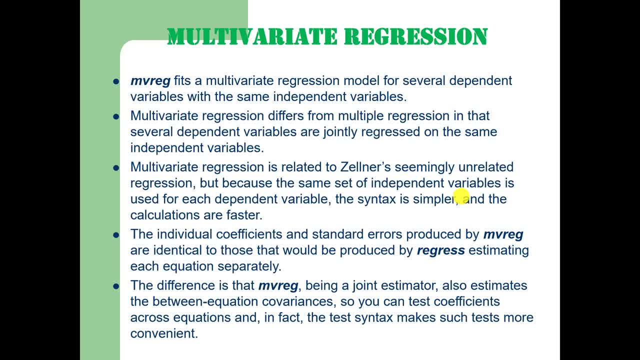 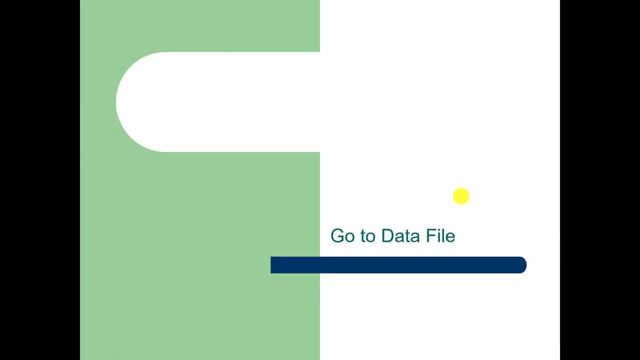 can test coefficients across equations and in fact, the test syntax makes such tests more convenient. In order to run or estimate multivariate regression, we will go to Stata file and we will use the mvreg command for regression- multivariate regression. So let us start. 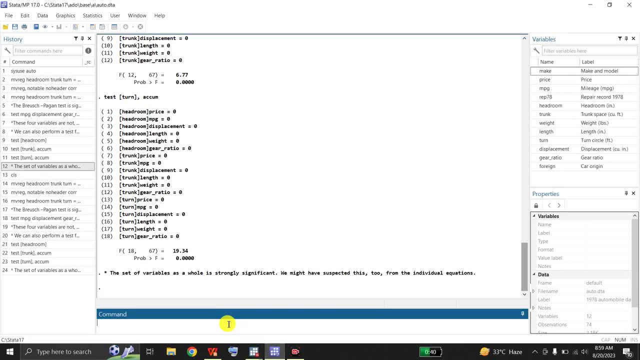 So here is my Stata file that I have already uploaded and this is a Stata example data set and I have opened this from the net, from the Stata, and now I will use the mvreg, that is, multivariate regression, using this file. First of all, I will give this command: mvreg. 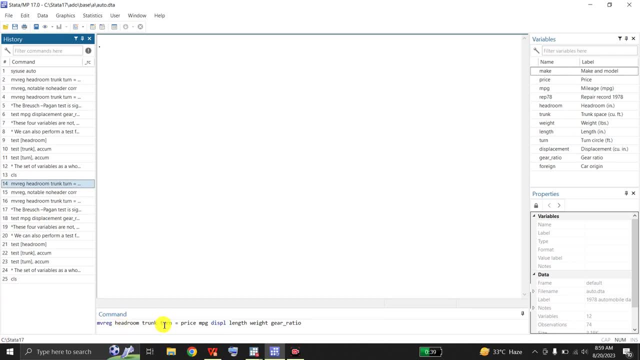 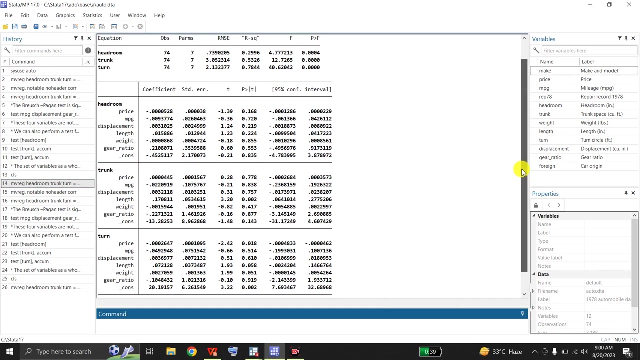 t, in which headroom, trunk and turn are the three dependent variables, and we will regress these three dependent variables on the set of independent variables on the right hand side, which include independent variables as price, mpg, displacement, length, weight, gear ratio. So by giving this command, the command is here, this is the command and these 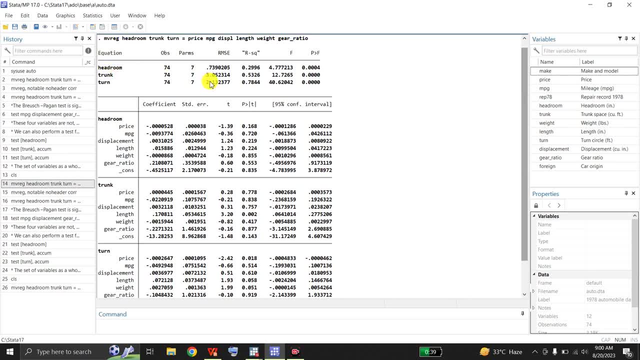 are the variables that we are going to use to do the regression. So we will use this command and we will regress these three dependent variables and we will the three individual equations related statistics: number of observations, parameters, root mean square errors: r squared for the three equations: f values and p values. These are the estimated. 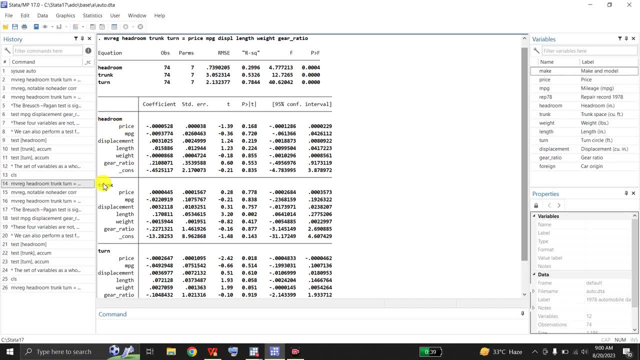 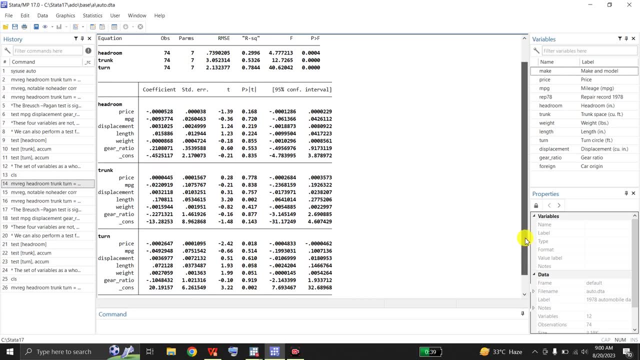 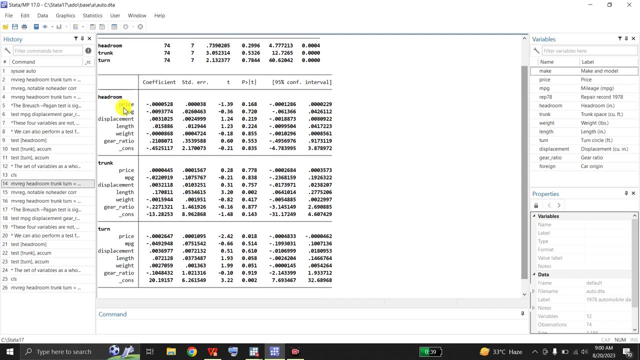 equations: This is for headroom, This is estimated equation for trunk and this is estimated equation for turn. So all the three dependent variables have been jointly estimated by the MV ray command and the same set of independent variables. These are the coefficients, These are the standard. 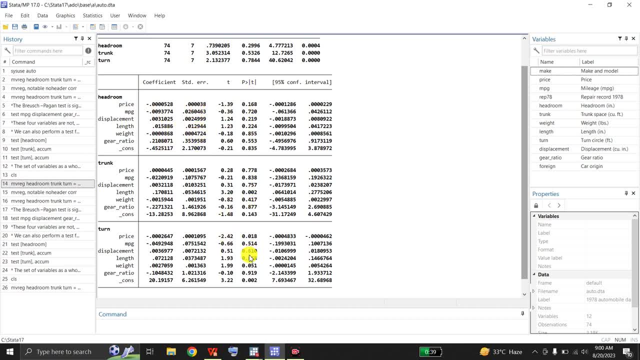 errors. These are the t values, These are the p values and these are the 95 percent confidence interval for the three individual equations, Since there are three joint estimation of the three individual equations and we may suspect that the residuals in the three equation may be. 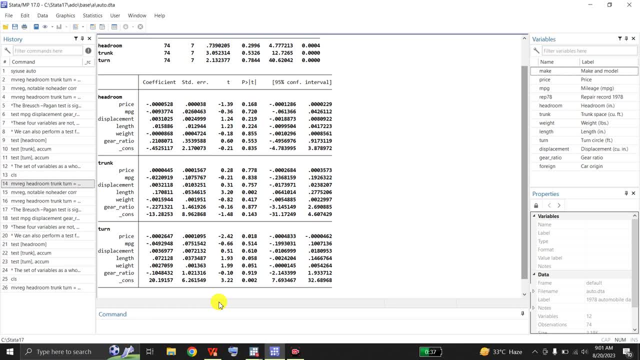 dependent on each other. So for that we may run a test and I will give this command. I ask Stata to give me correlation matrix of the residual of the three equation, but don't give me the estimated equations in tables and headers. So here is the correlation. 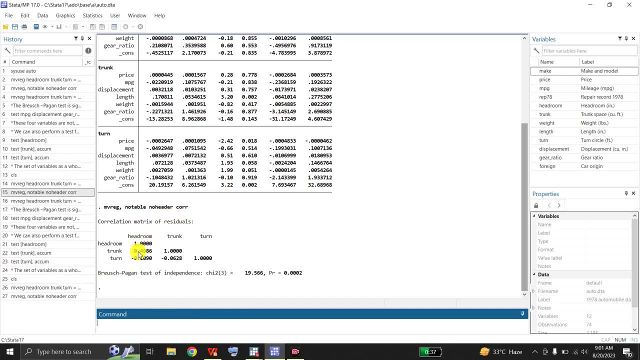 matrix of the residuals of the three. equation: The, the, the. the correlation between the headroom and the trunk residuals is 0.49, for the headroom and turn is minus 0.109 and for the trunk and turn is minus 0.06. and here is the bruspegan test of. 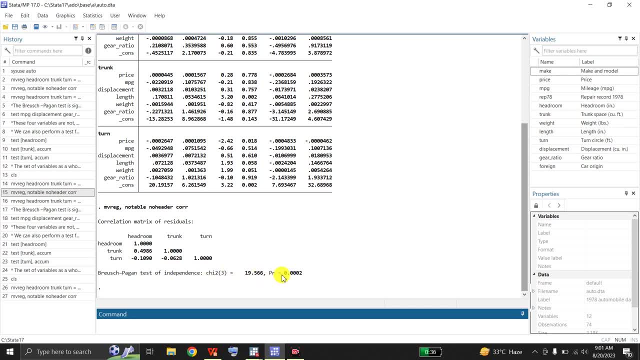 independence based on chi-square test, and its relevant p value is 0.002. so this bruspegan test is significant and we conclude that the residuals of the three equations are not independent. they depend upon each other. we can also produce the same results by this equation, by this command. 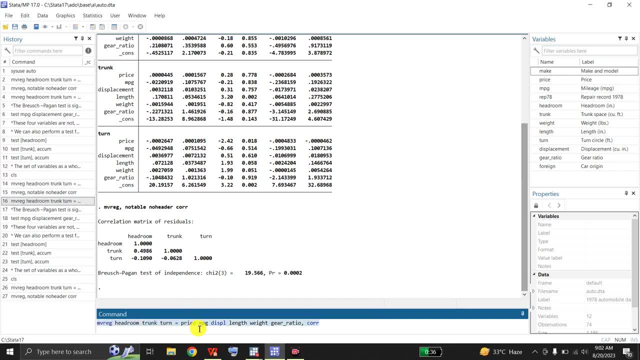 in which the command from mv rec up to gear ratio is the same as i give it here above to estimate the three equations. but now i follow this by comma and correlation, so it will estimate for me the three individual equations on the same set of independent variables. 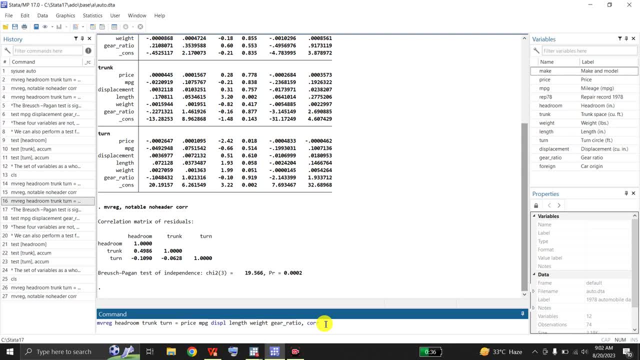 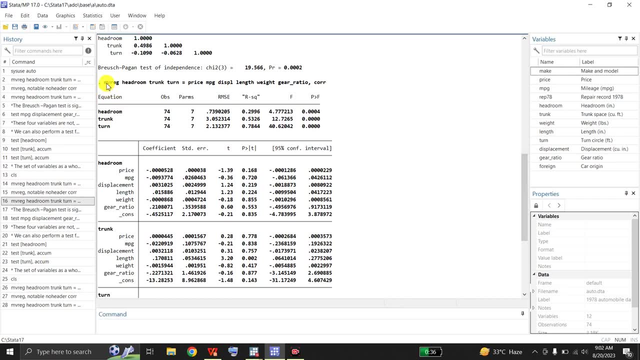 and it will also give me a correlation coefficient of the residuals of the three equations. so the same result has been produced now. now this is the mv rec headroom trunk turn. that equals price, mpg, displacement, length, weight, gear ratio, comma and correlation. so it means the stata has estimated. 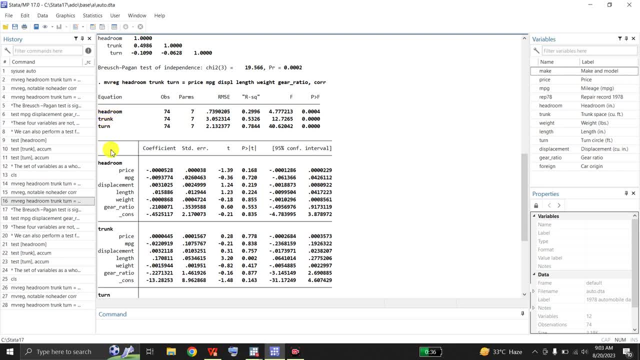 these three equations, for the three individual equations. so it will estimate for me the three values. so this result has been executed by the same set of independent variables. and finally, i will create a, finally a correlation coefficient matrix for the residuals. here is the correlation matrix of the residuals of the three equations. so i frame this: 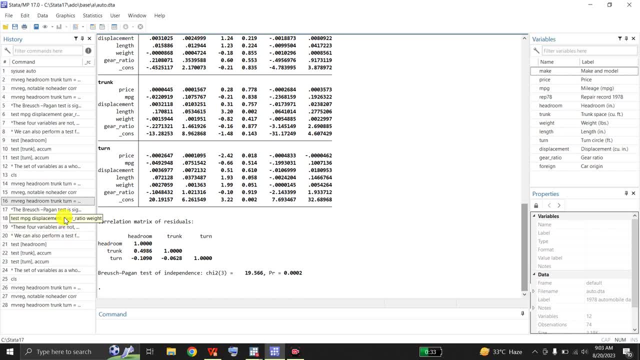 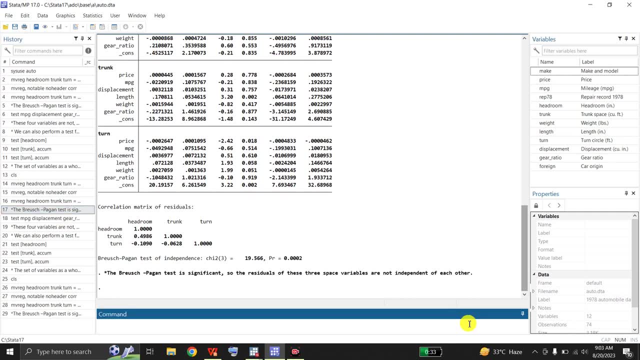 the correlation matrix will give me the correlation for the three equations. so, based on this p, we may use this result. the bruspegan test is significant because the p value is less than 0.05. so the results, so the residual values between we have here are 0.00 거리를 left and which is the proportion between each of these values here is 50 odd or 50. That is 60. So next will be the result, based on the relation between the three equations, based on the two equations as well, that we will make this close to 10 Ramen. 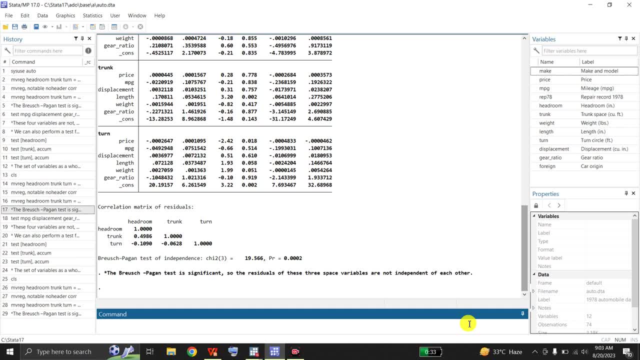 So the residuals of these three space variables are not independent of each other. They depend upon each other. Let me test a number of coefficients at the same time that these coefficients are equal to zero. So test MPG, displacement, gear ratio and weight. 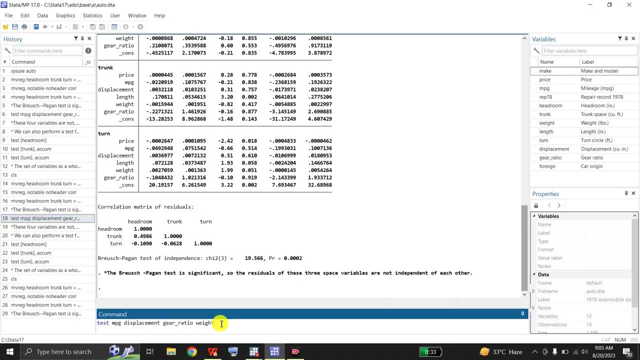 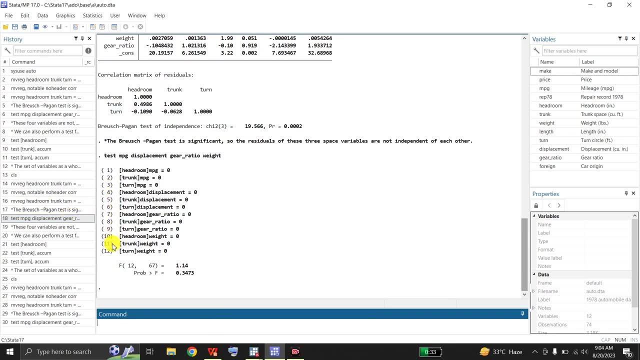 Test jointly that the coefficient for MPG displacement, gear ratio and weight is equal. So there are 12 coefficients, 3 equations and there are 4 variables: MPG, displacement, gear ratio and weight. So 4 variables and 3 equations. 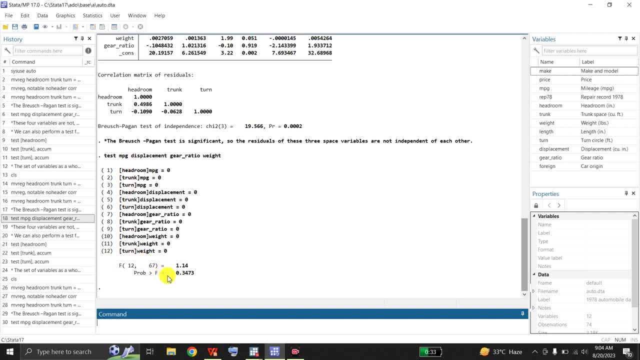 So the total number of coefficients are 12.. And the null hypothesis is that these coefficients are jointly equal to zero. in various equations, That is, Across equation, the coefficients of these four variables are equal to zero. So, based on this F value, the P value is 0.3473. 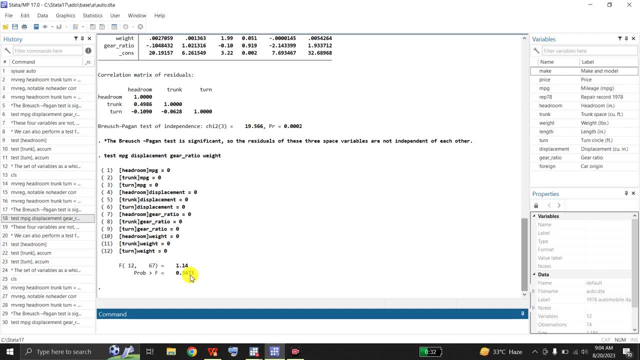 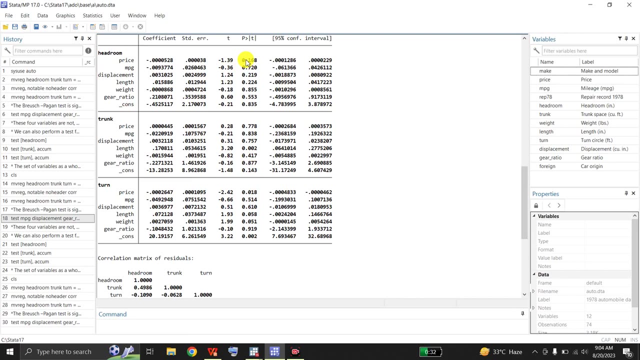 And we fail to reject the null hypothesis and we conclude that these coefficients across equations are equal to zero, Because we can also guess the same thing from this equation. Majority of the majority of the coefficients are insignificant In overall. in the 12 coefficients, only one coefficient is significant. 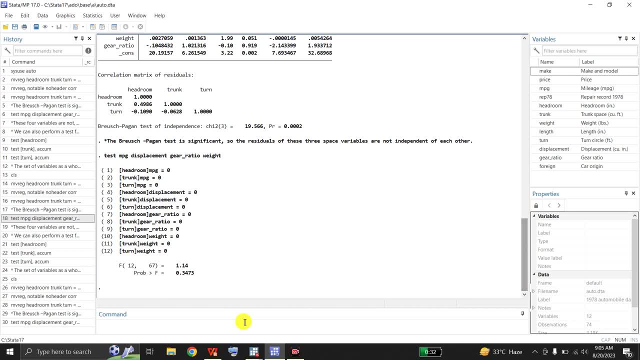 So on the basis of this test, we conclude that the coefficients of these four variables in three equations are jointly not different from zero. So we can also, We can also. So these four variables are not as a group significant, And we also saw this. 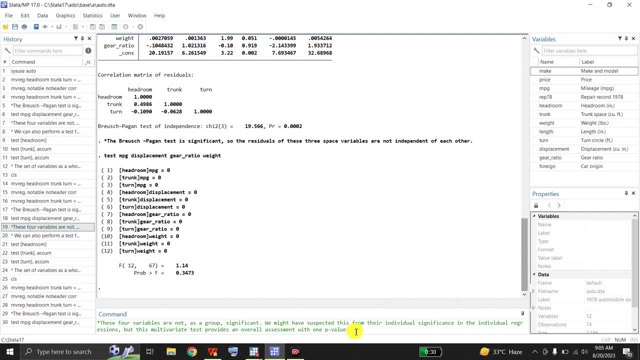 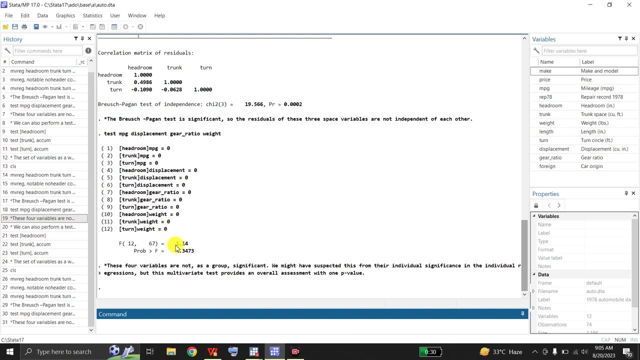 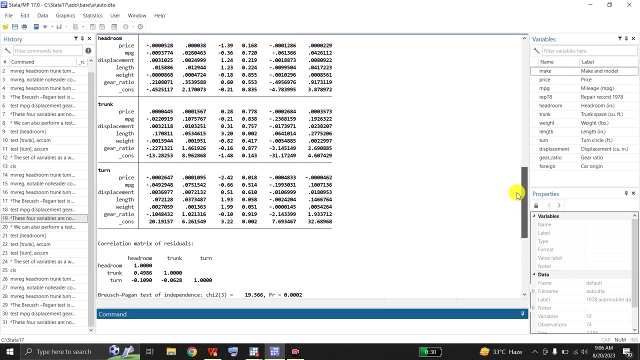 We suspected this from their individual significance in the individual regression, But this multivariate test provides an overall assessment with one P value And this is the one P value. So jointly, the as a group, These four variables are not significant And we can guess this from these coefficients. 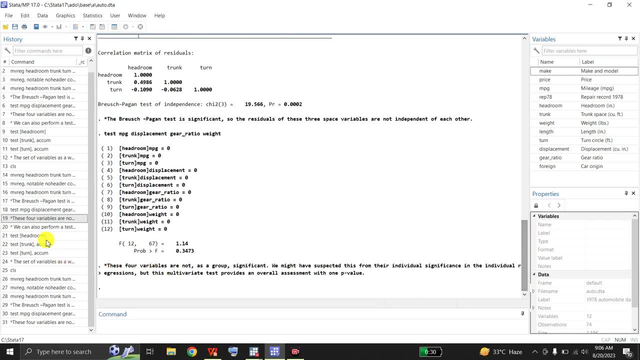 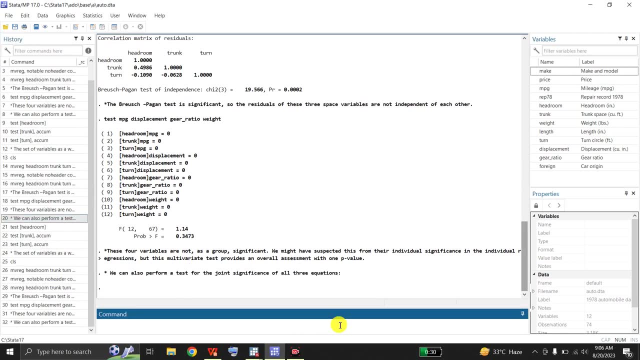 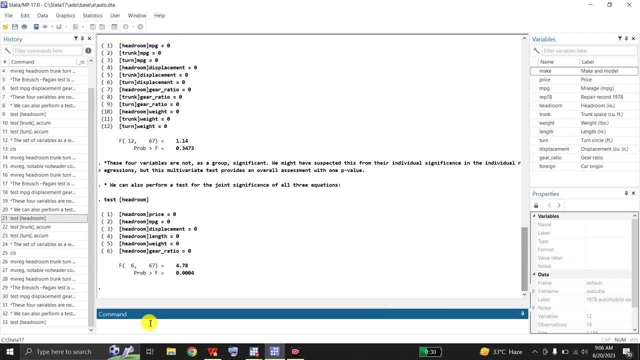 We will use here. After this, we can also perform a joint significance test for all the three equations, And for that we can use these commands. This is test for the head rooms And this is for the, For the, For the. 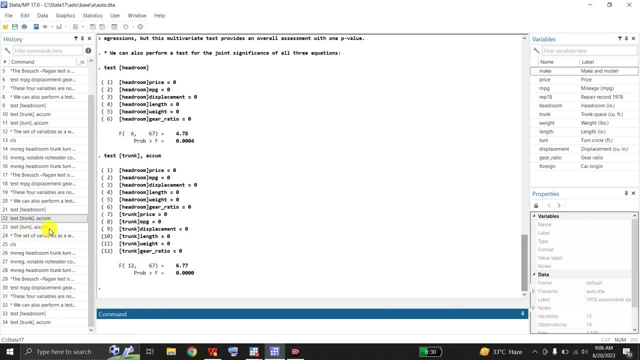 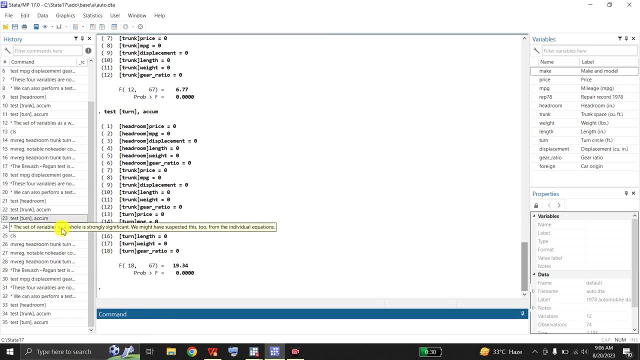 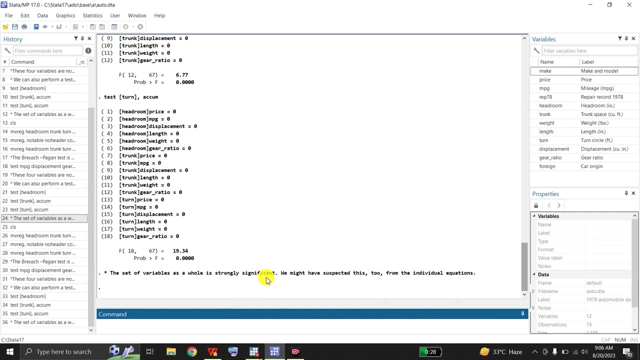 Turn. So we can guess, based on the P values of these three equation, That the set of variable is a whole is strongly significant. The set of variables is a whole is strongly significant. We might have suspected this too from the individual equations and from the individual equations. 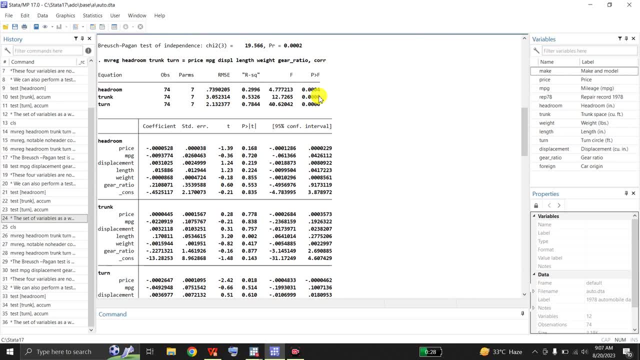 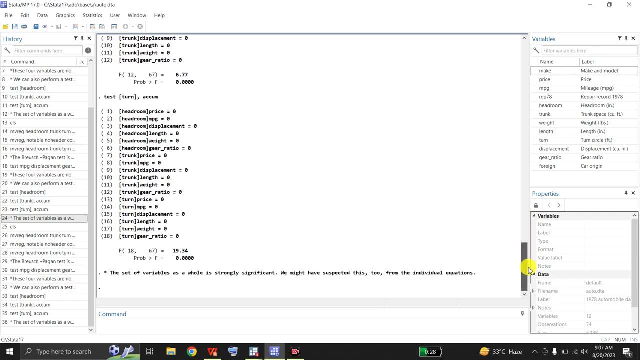 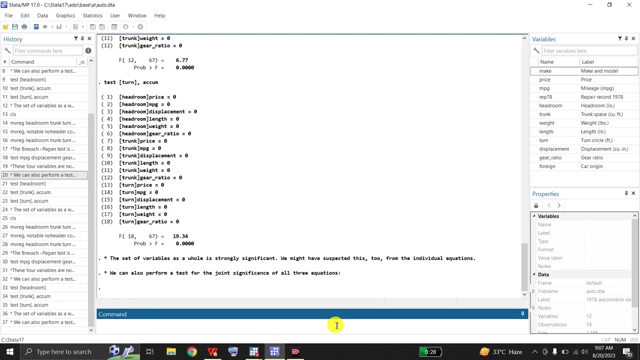 We saw earlier that these f statistics, their p values, are significant and we have proved the same thing with this joint test of. we can that earlier we said we can perform a test for the joint significance of all the three equations and we showed that by this equation that the set 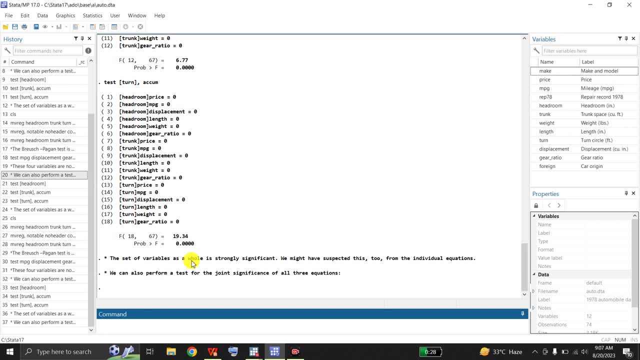 of the variable as a whole is strongly statistically significant, and this we suspected earlier, also from the p values. so, ladies and gentlemen, this is very interesting and we found difference between multiple linear regression model and multivariate regression. and the difference between multiple linear regression model is that in that regression, 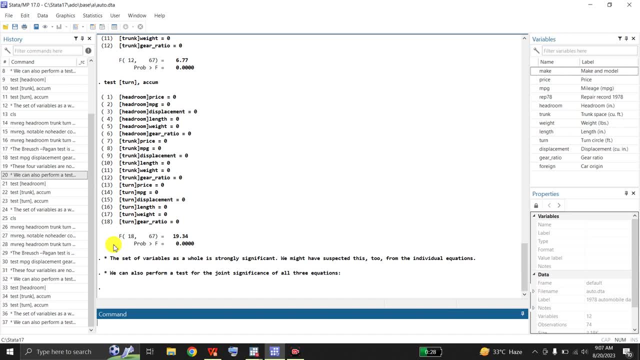 we estimate or we regress one dependent variable on a number of independent or explanatory variables. but in case of multivariate regression, more than one dependent variables are jointly regressed on the same set of independent variables on the right hand side and we can test assumptions of a joint significance of